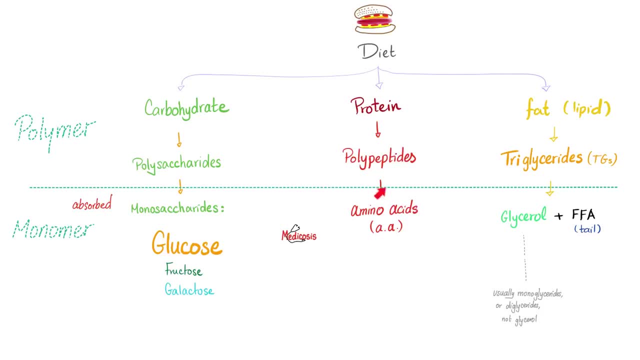 then oligopeptides, then dipeptides, and then amino acids. How about a monopeptide? Well, there is no such thing. Shut up, A monopeptide is one amino acid, Fats or lipids, triglycerides- these are the big ones, And then glycerol and fatty 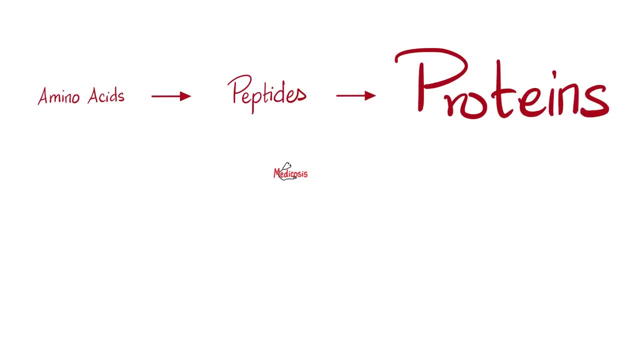 acid. these are the small ones. Here are amino acids. They become peptides and then they become proteins. These are the macromolecules. These are the micromolecules: Polymers, monomers. So while walking down the street, how can I pick an amino acid? How can I recognize the 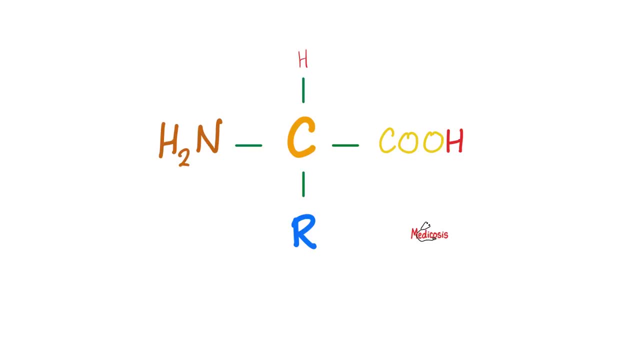 doofus. All right, The doofus will have an amino group on one side and a carboxyl group on the other side, And you have a carbon in between. This is called the alpha carbon. This carbon is attached to R, which is the side chain, And just to balance it. 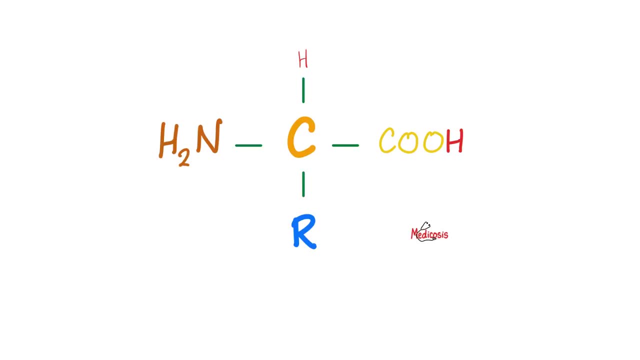 you have to add an H here, because carbon requires four bonds: Amino group here, carboxyl group here. This is the side chain, or the R group, And this is the one that determines the properties of the amino acids, Chemical properties that is. Does the order matter? Like should I write the amino? 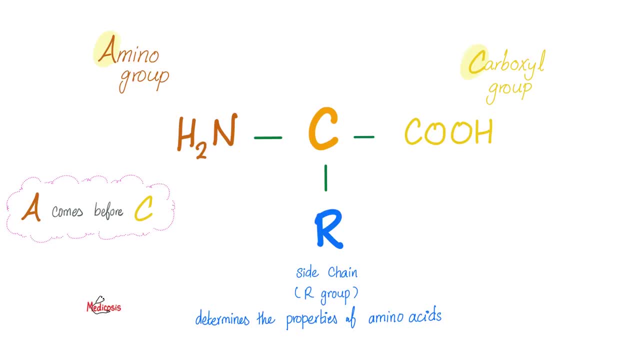 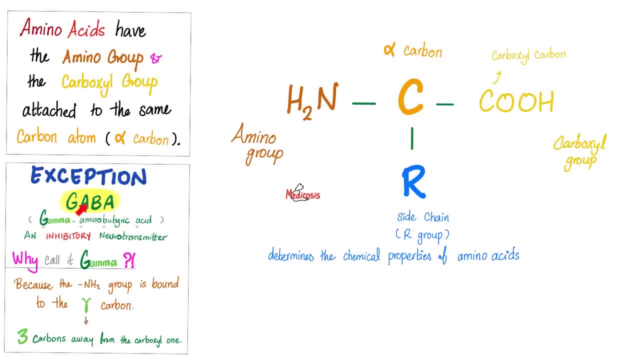 This is GABA. GABA stands for what? Gamma Amino Butyric Acid. Say it one more time, because it was so beautiful: Gamma Amino Butyric Acid, Gamma, You know why we call it gamma? Yep, indeed, Because it's a gamma carbon, which is three. 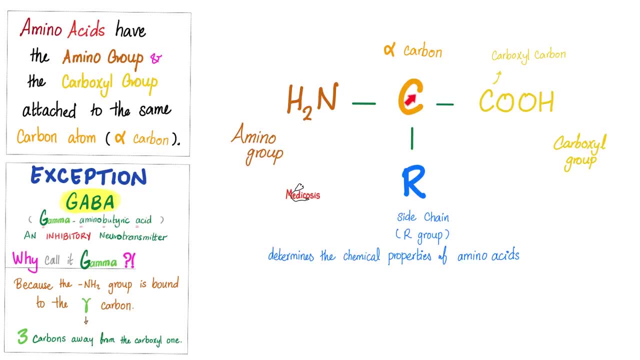 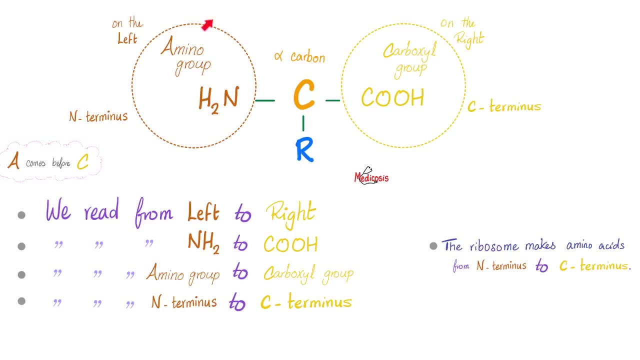 carbons away from the carboxyl one. So after the carboxyl you have alpha and then you have beta and then you have gamma carbon. In English we read from left to right. Same thing with amino acids. We read from the amino group towards the carboxyl group. Why do we care? Because this is 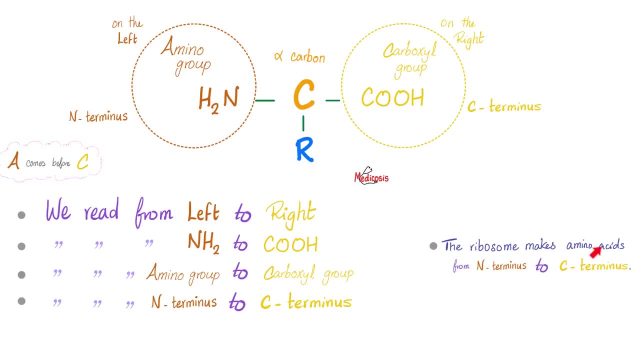 the order of the amino acid coming out of the freaking ribosome on the rough endoplasmic reticulum. if you remember, The ribosome makes the amino acid come out of the carboxyl group, The N-terminus first, before the C-terminus. That's why we care. Let me ask you a question. 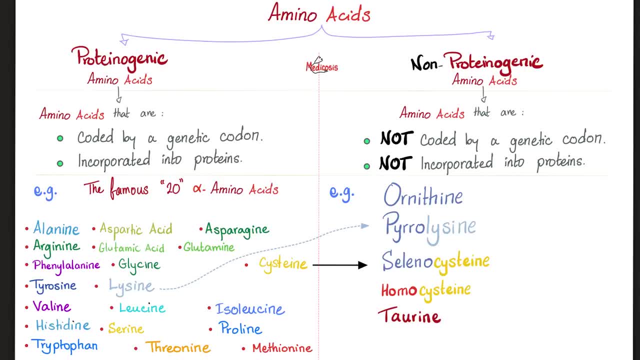 How many amino acids do we have in our bodies? Oh, I know Medicosis. My biology professor told me that we have 20 amino acids only. Shut up. Your biology professor is myopic, no pun intended. The 20 amino acids that you're talking about are only the proteogenic amino acids. You have other. 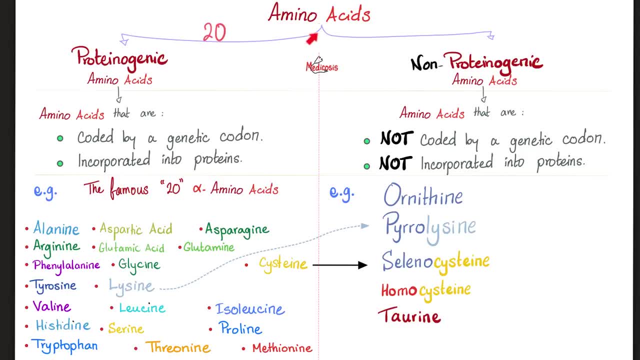 non-proteogenic amino acids in your freaking body. But what's the difference? Proteogenic amino acid, just by the name. look at the name proteogenic. So they will make proteins. Oh yeah, they are incorporated into proteins. 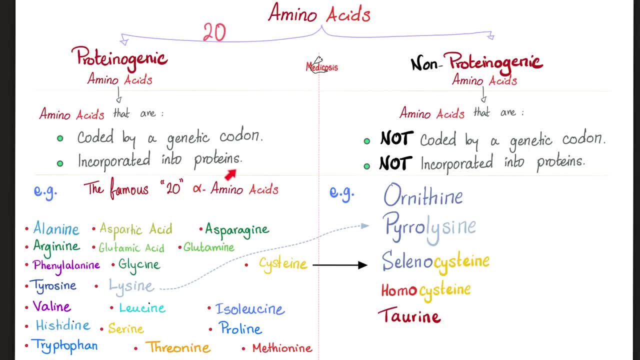 Amino acid. an amino acid, another amino acid. make them into peptides and then proteins. They are also coded by a genetic codon. Remember these three lovely nitrogenous bases. What are these 20 amino acids that your biology professor told you about? Yeah, 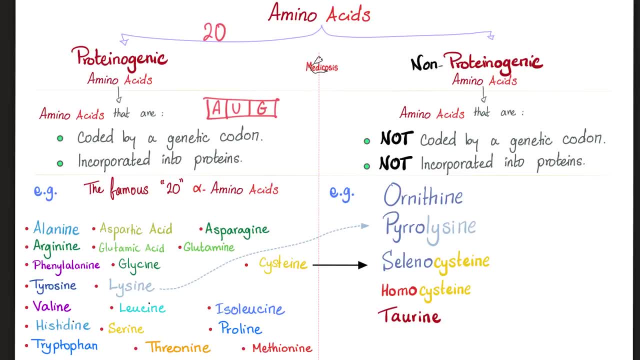 the famous alanine, aspartic acid, asparagine, arginine, glutamic acid, glutamine. So you have the amino acid aspartic acid, aspartic acid, asparagine, arginine, glutamic acid, glutamine. 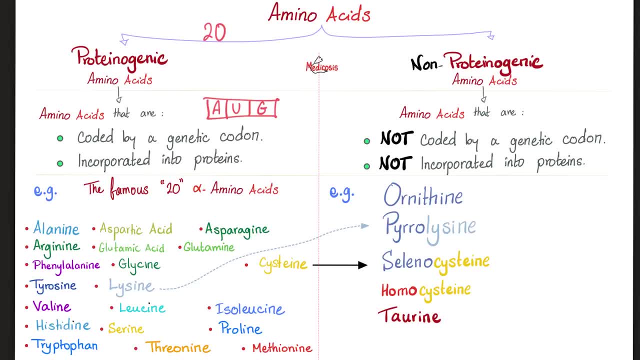 Phenylalanine, glycine, tyrosine, lysine, valine leucine, isoleucine. You need to remember these three together: Valine leucine, isoleucine, histidine, cysteine, serine, proline, tryptophan. 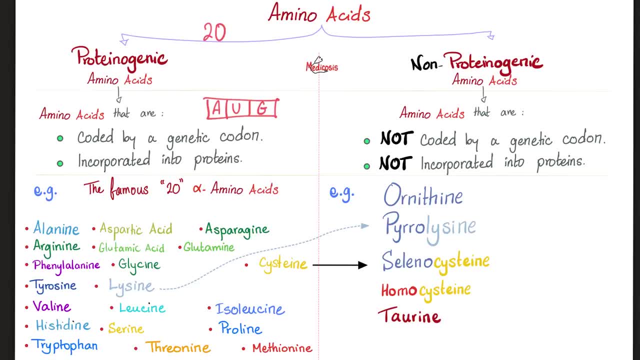 threonine methine- My favorite, because it gives your Uncle Sam a methyl donor. How about the non-proteogenic? All right, they are not coded by a codon, They are not incorporated into proteins, but they exist. 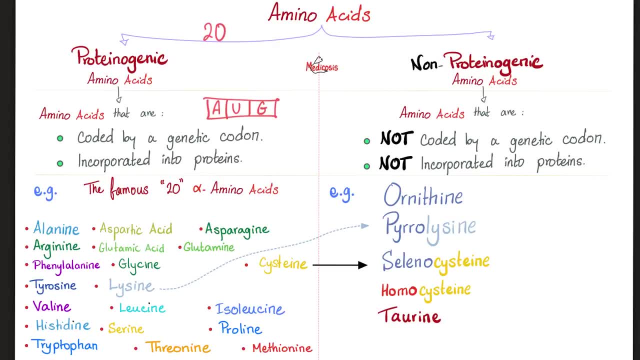 Such as ornithine. if you remember your urea cycle, Pyrolycine- where the flip did you get pyrolycine from? From lysine Selenocysteine. where do you get from From cysteine Selen means. 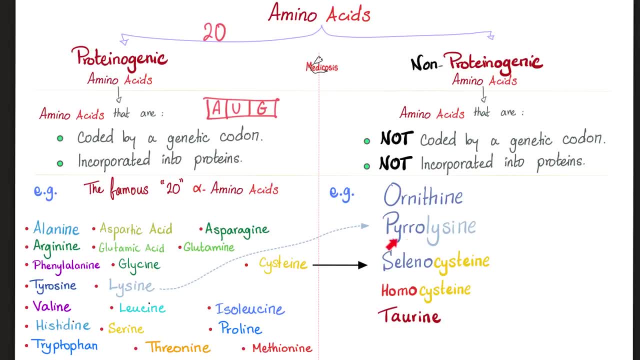 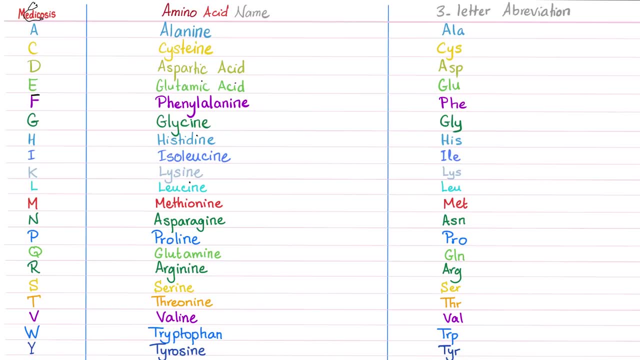 selenium Pyro, because it contains pyroline ring or pyroline side chain. Where did homocysteine come from? From cysteine? Do you remember the coagulation factors? Yeah, each one had a name and a number. Okay. 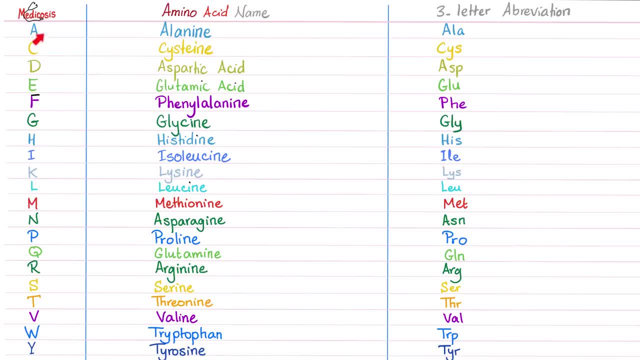 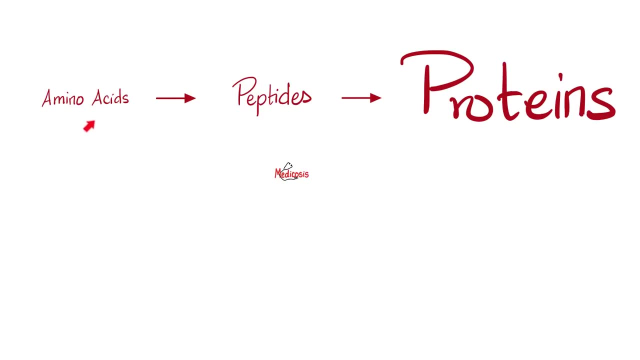 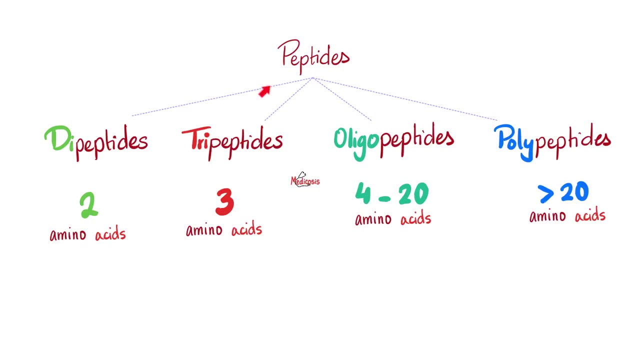 Each one has a name, a one-letter abbreviation and a three-letter abbreviation. You need to memorize all of this. As you know, amino acids are the small ones, micromolecules, then peptides, then the big ones, proteins. But not all peptides are created equal. We have dipeptides, tripeptides. 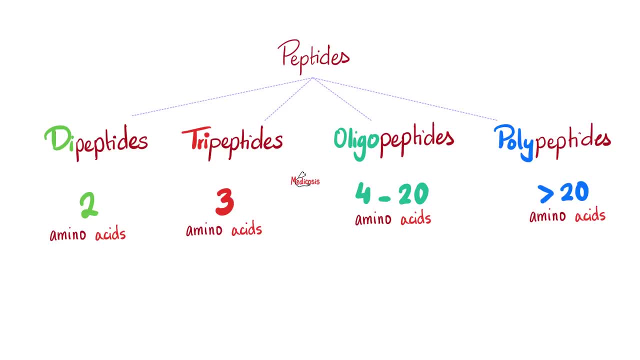 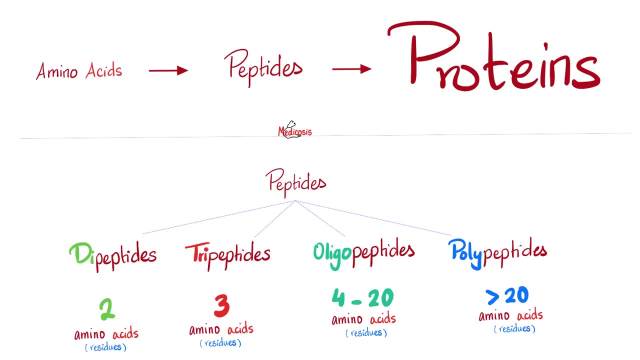 oligopeptides and polypeptides. Di means two, so dipeptides two amino acids, Tripeptides three amino acids, Oligopeptides from four to twenty, Poly more than twenty. Therefore, in all honesty, it goes like this: Amino acids followed by dipeptides followed. 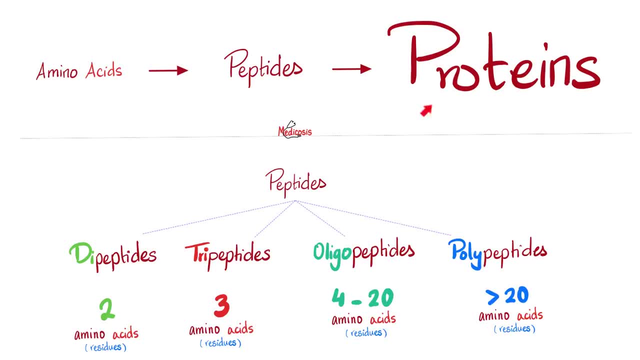 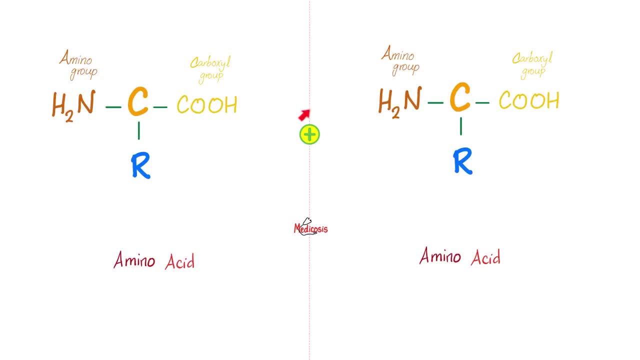 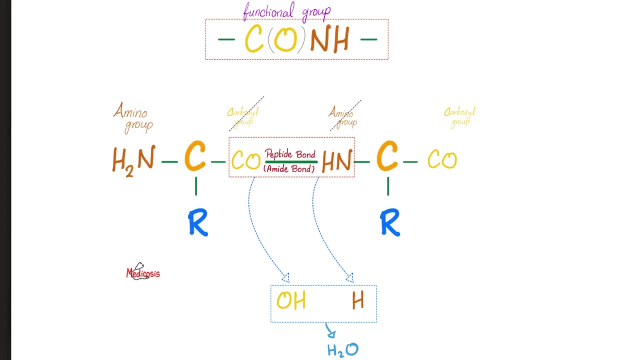 by tripeptides, oligopeptides, polypeptides, then proteins. Pause and review. An amino acid plus an amino acid equals dipeptide. How do we join them together Through a peptide bond? This was COOH. Say goodbye to the OH. Now you have CO and stop. And then this was: 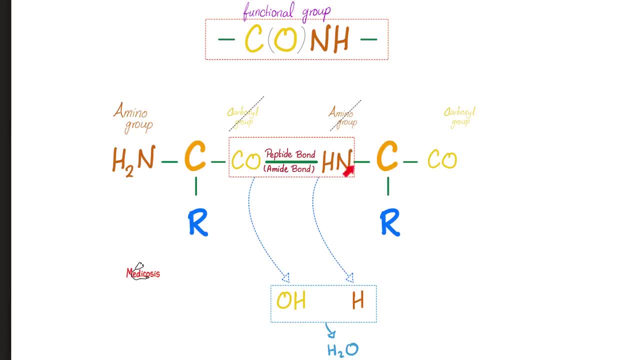 NH2.. Say goodbye to 1H. So you're only left with NH2.. So you're only left with NH2.. So you're only left with OH and H. Alright, Then what's the functional unit here, CO, HN or NH? So, 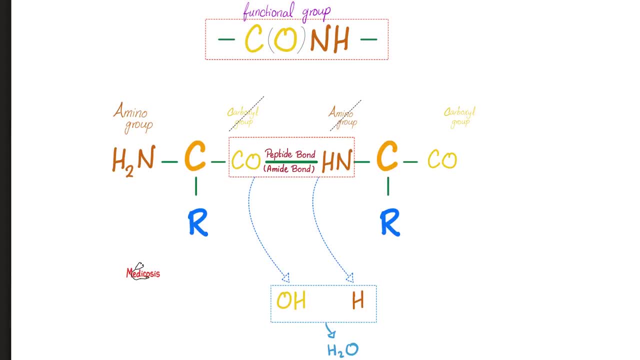 CONH is the functional group. What kind of bond is this? Peptide bond, aka amide bond. What's gonna happen to the OH and the H? You're gonna combine them together to make water. So peptide bond formation looks like this: Amino acid number one plus amino acid number. 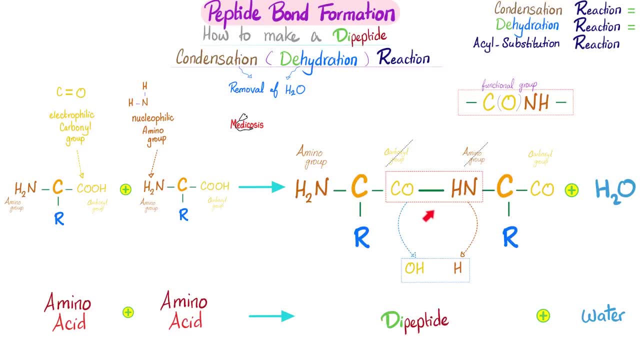 two, and then boom, combine them together. This is your beautiful peptide bond and this is the water. What do you call this Dipeptide? What kind of reaction is this? Well, any reaction that removes water is a dehydration reaction. Any reaction that removes water is a condensation. 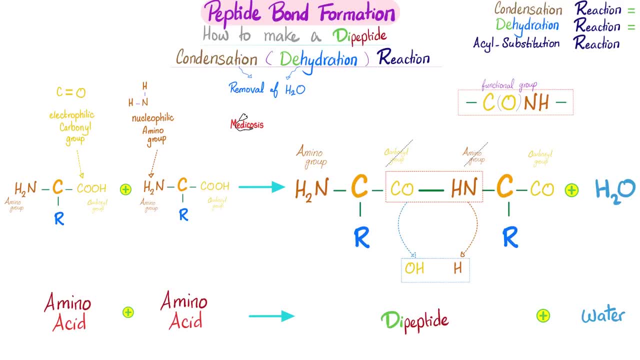 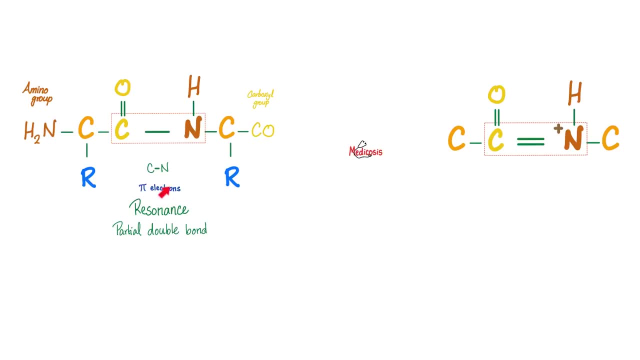 reaction. You can also consider it an acyl substitution reaction. CONH is the functional group. Between C and N there is a pi electrons. Therefore there is resonance. What the flip is resonance. Resonance means magnification. They become more robust. Why? Because this is a partial 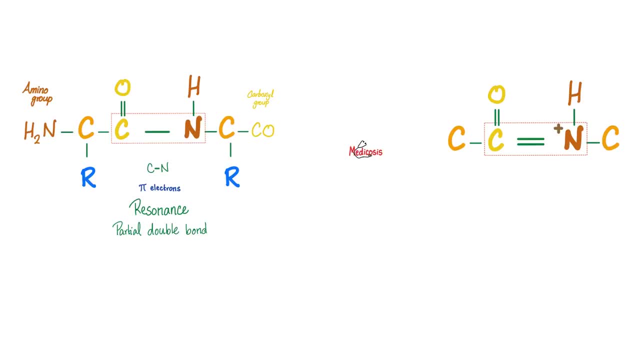 double bond. So this is a partial double bond. So this is a partial double bond. So this is a double bond Like this: That's double, Oh, but the N has to be N plus, This bond is the peptide bond. 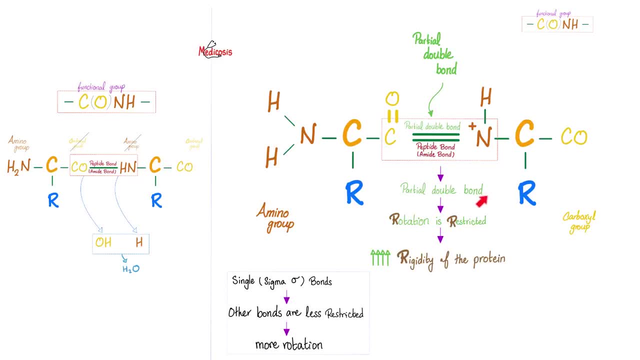 or amide bond, Can you describe it? Sure, It's a partial double bond. Therefore, rotation is restricted. Why? Because it's a double bond. You cannot rotate around a double bond And if you cannot rotate you are rigid. Contrast that with these single bonds. These are sigma bonds, Sigma. 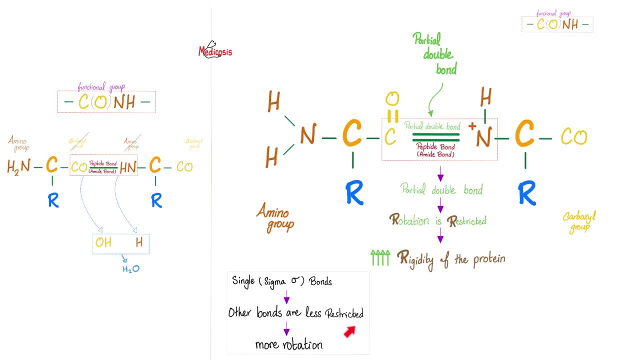 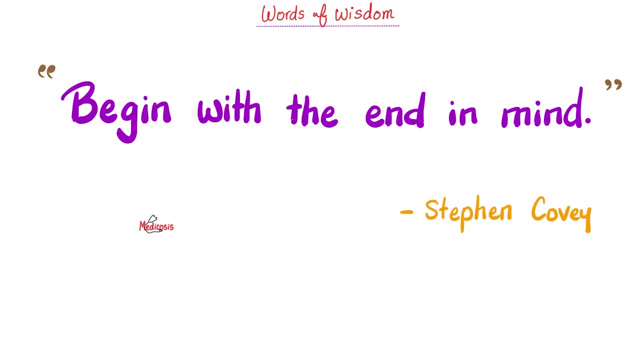 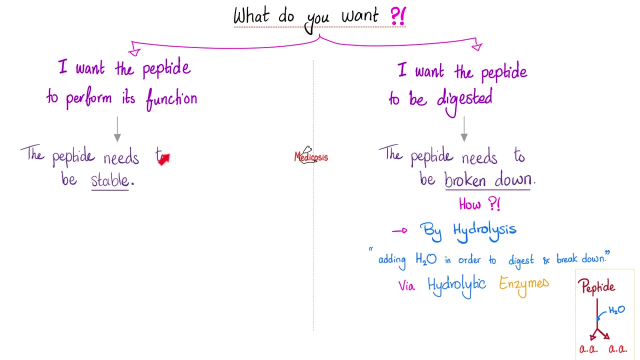 is single, Signal is sigma and sigma is single. They are less restricted Hashtag, more rotation. Got some swirling action going. Dr Stephen Covey said: begin with the end in mind. Ask yourself, what am I trying to achieve? Oh, I want the peptide to performance function. Sure, Then the 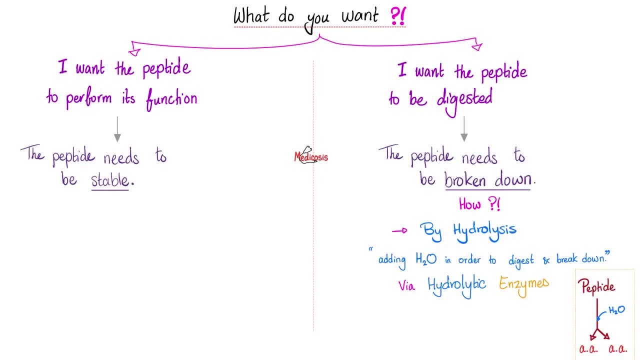 peptide needs to be stable, Right. But if you have a different goal in mind, I want the peptide to be digested. Now the peptide, it needs to be broken down. How do I break a peptide By hydrolysis? 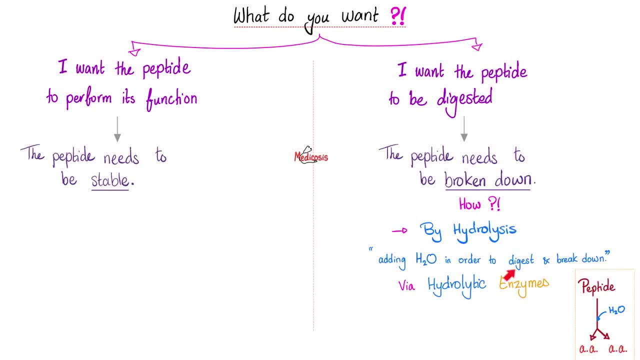 by adding water. So hydrolysis is adding water in order to break down something. Who does that? A hydrolytic enzyme? Well, no, duh, You see that That's a peptide. When you add water to the peptide, oh, you break it down to amino acid. Hashtag hydrolysis. Hashtag hydrolytic. 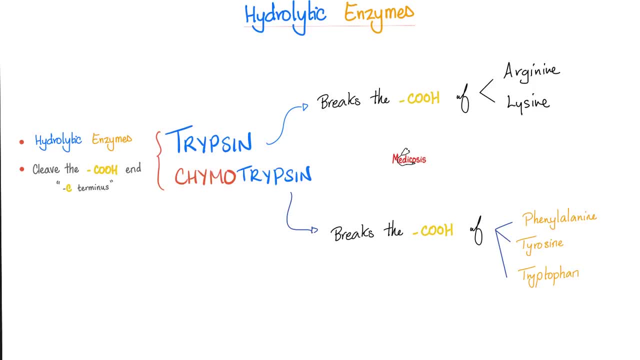 enzymes. Can you give me examples of these hydrolytic enzymes? Sure, Trypsin and chymotrypsin. They are hydrolytic enzymes that cleave the carboxyl group. They cleave the C-terminus. 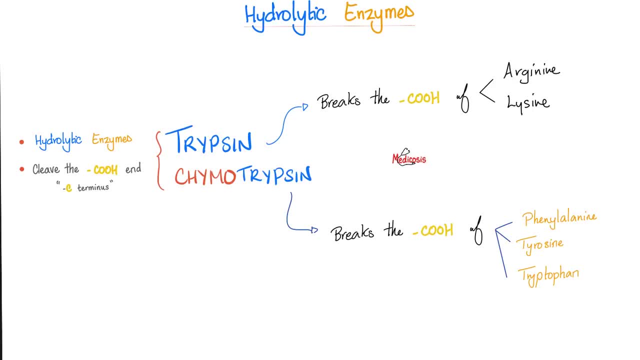 And this involves both of them. However, what's different about trypsin is that it breaks the carboxyl of arginine and lysine. However, it breaks the carboxyl of arginine and lysine. However, chymotrypsin, it breaks the carboxyl of other amino acids such as phenylalanine, tyrosine. 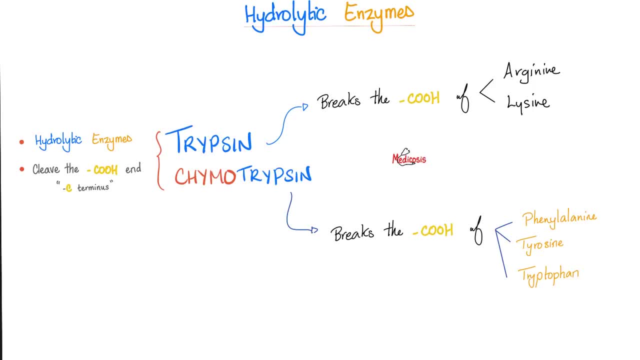 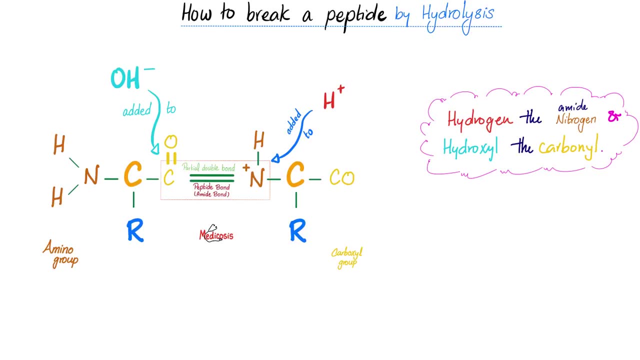 and tryptophan. These are the similarities, These are the differences. How to break a man? I mean how to break a peptide. You break it by hydrolysis. What do you mean by hydrolysis? Add water in order. 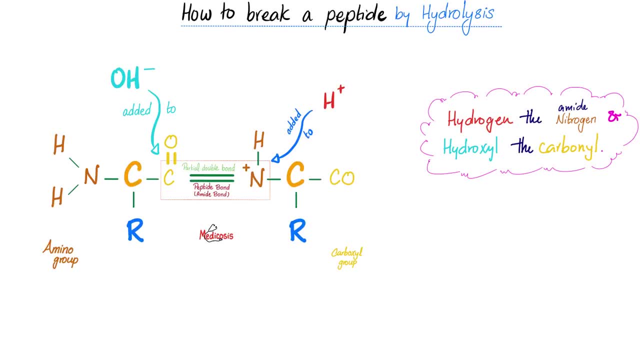 to break down. So here is H and OH. This is water. H plus OH is water. Add the H here, Add the OH here. This will become COOH and this will become NH2.. You added hydrogen. You added hydrogen to the nitrogen and you added hydroxyl to the carboxyl. I love it. It has a good 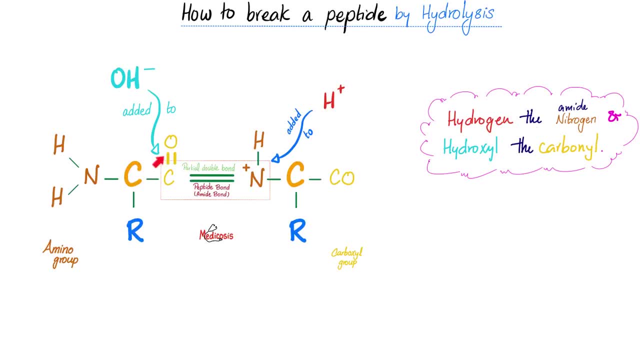 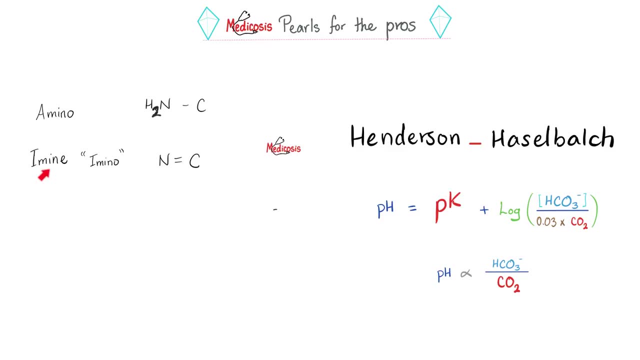 ring to it. Add hydrogen to the nitrogen, Add hydroxyl to the carboxyl And this is how you break a peptide. Some pearls for the pros. What's the difference between amino and amine? or amino? Okay, amino is C bound to N with a single bond. But look at amino double bond. Don't forget the.